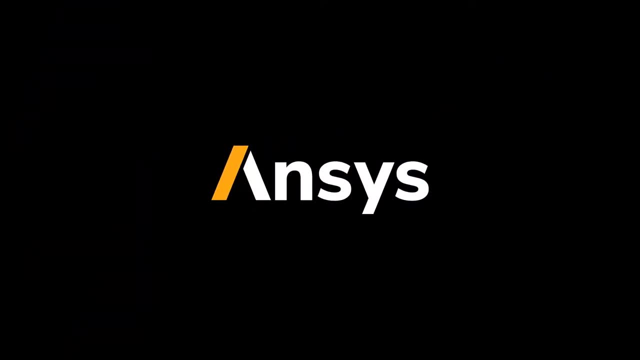 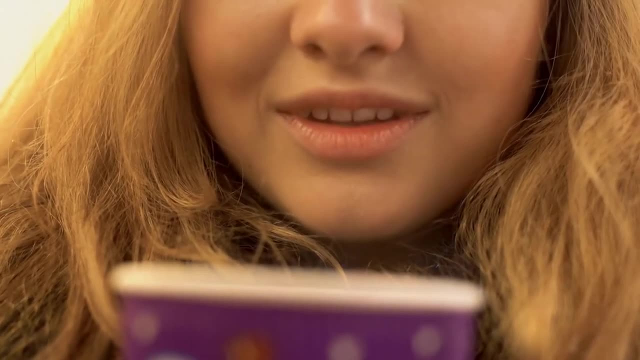 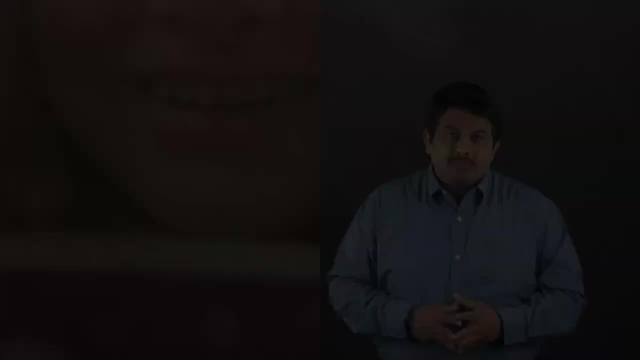 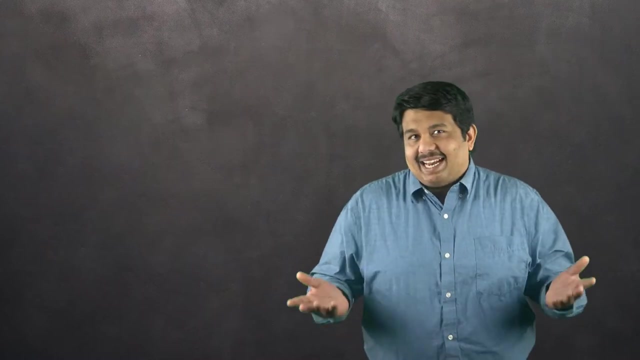 Have you ever noticed how blowing on a hot beverage, say a cup of coffee, cools it down much faster than if you just left it on the table? What you are unconsciously doing is employing forced convection to cool your coffee faster. Let's take a deeper look at what 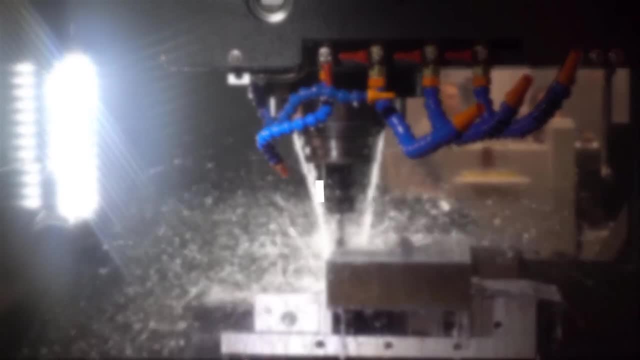 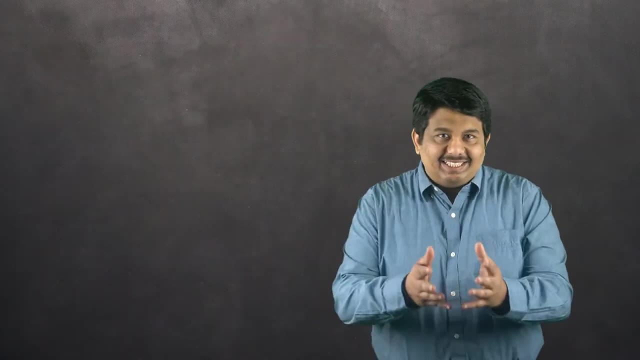 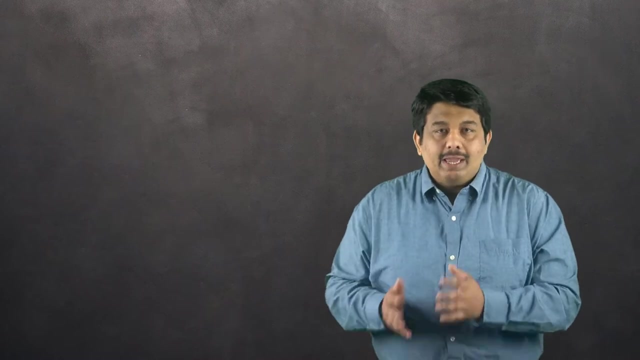 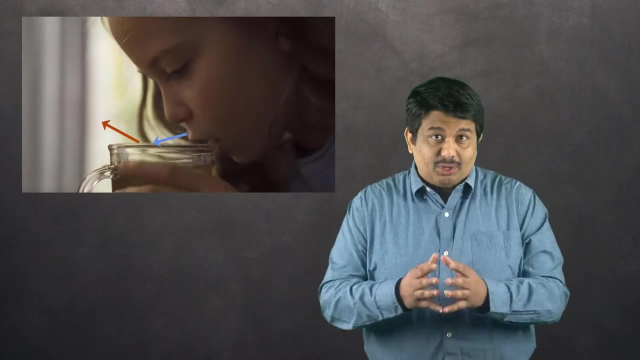 forced convection is all about. Convection is the mode of heat transfer, where energy is transferred to or from a cold body or a hot body by fluid motion. Back to the coffee example. The air you blow extracts heat from the coffee and convects it away. 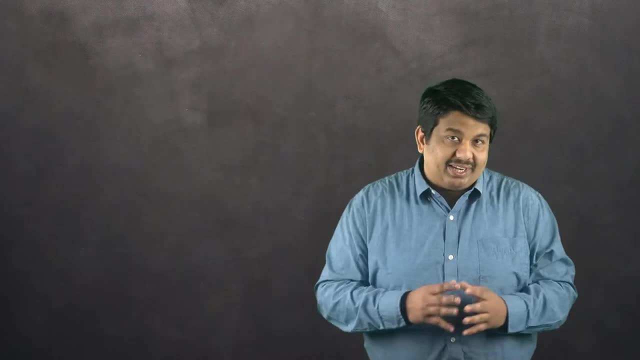 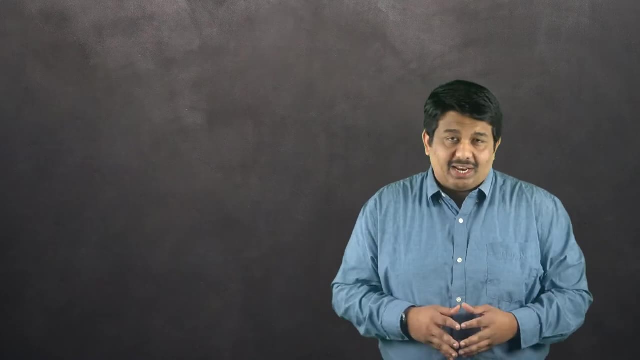 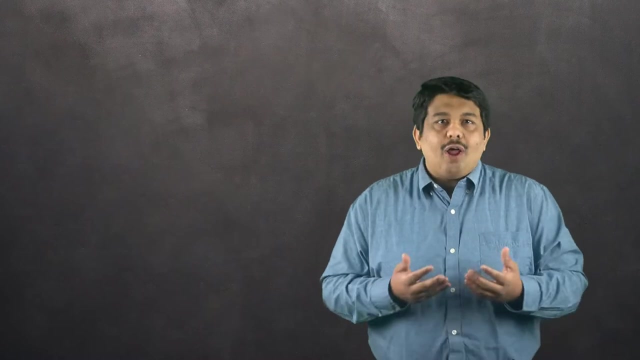 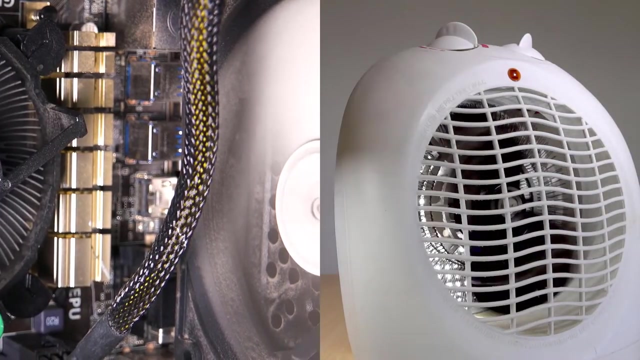 from the mug. Based on how the fluid flow is created, convection can be classified into natural or forced convection. In forced convection, the fluid flow is generated by external means, ie by a fan or because of an object's motion. cooling of electronic components: localized space heaters are a 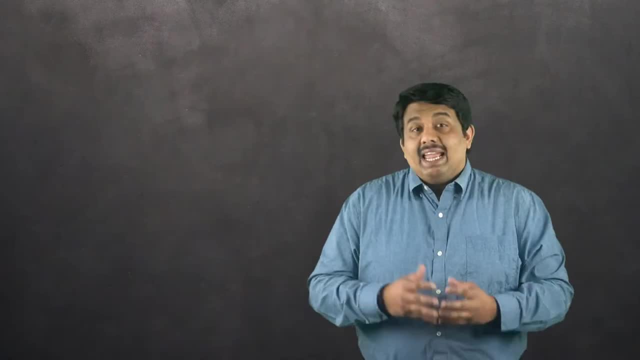 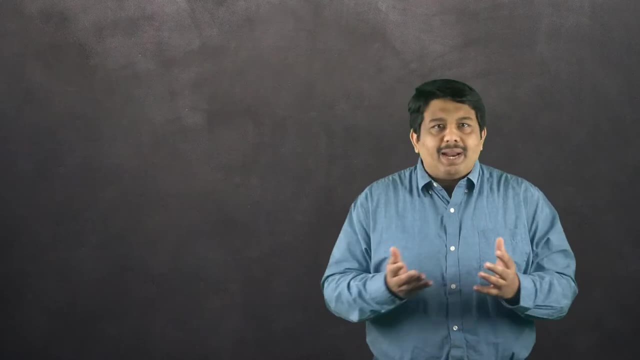 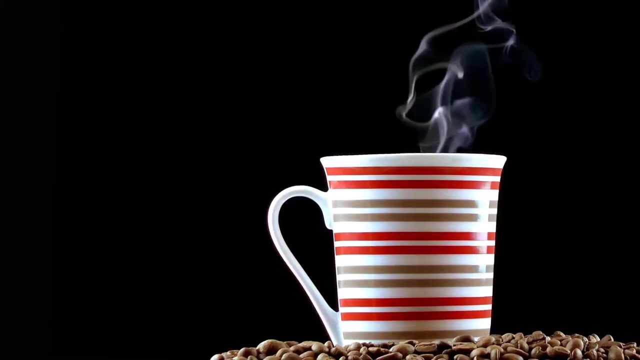 few examples of forced convection. In natural convection, a fluid flow is created because of buoyancy forces caused by temperature gradients due to the energy transfer between the body and the surroundings. Cooling of a hot coffee left on a table, heating a room through beaters are examples of heat. 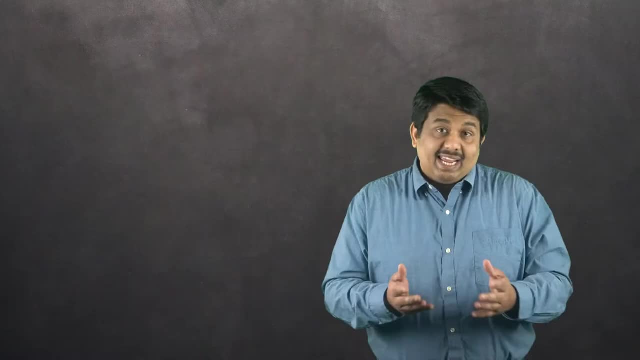 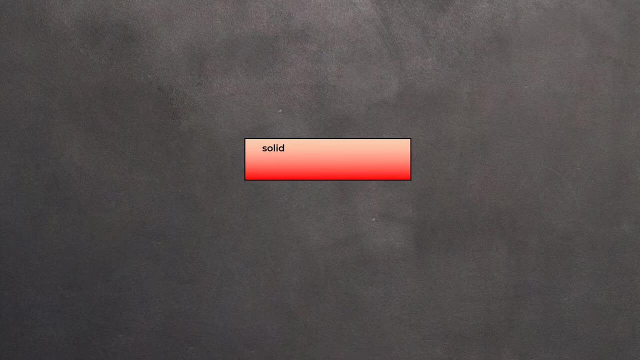 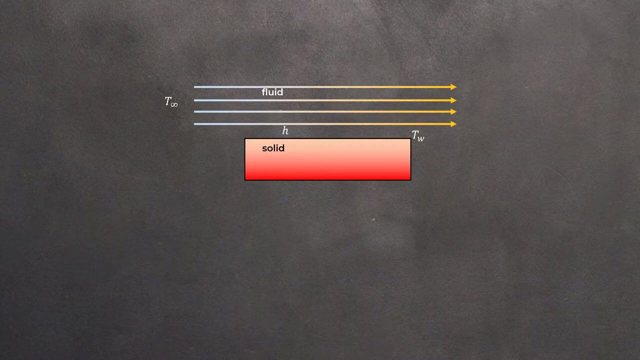 transfer via natural convection. In this course, our focus will be on forced convection. Consider a hot drink: If the incoming fluid is at temperature T-infinity and the heat transfer coefficient is H. according to Newton's law of cooling, the convection heat flux can be calculated using the following: 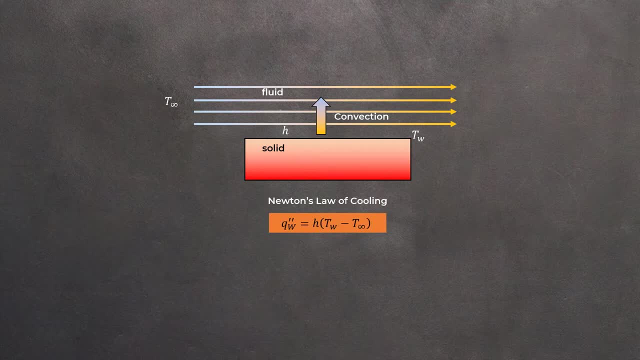 equation. At the surface of the plate there is no fluid motion due to the no-slip condition, and therefore there will be only conduction from the plate into the fluid, which is calculated using the Fourier's law as shown here. Neglecting radiation, these two fluxes must be equal at the wall and, as a result, we get: 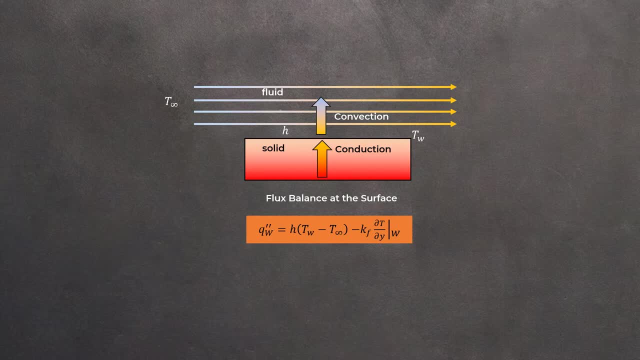 the following flux balance: Here Q'' is a local heat flux and therefore H is generally referred to as the local heat transfer coefficient. In general, heat transfer is a function of space and heat transfer. If the heat transfer coefficient is at an angle of H, then the heat transfer coefficient 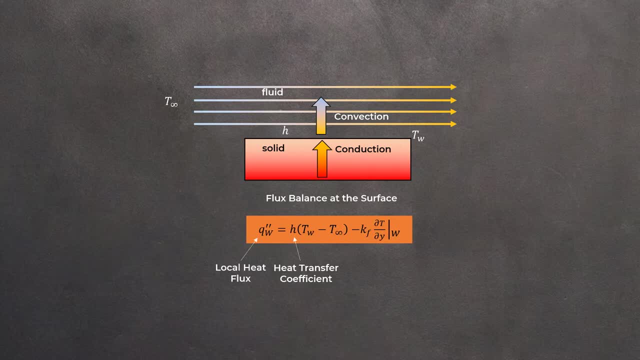 is equal to the local heat transfer coefficient. In general, heat transfer is a function of space, and heat transfer coefficient as well, and hence the heat transfer coefficient will vary over the surface. For engineering estimates, however, the averaged value of heat transfer coefficient for a surface can be defined as shown here. 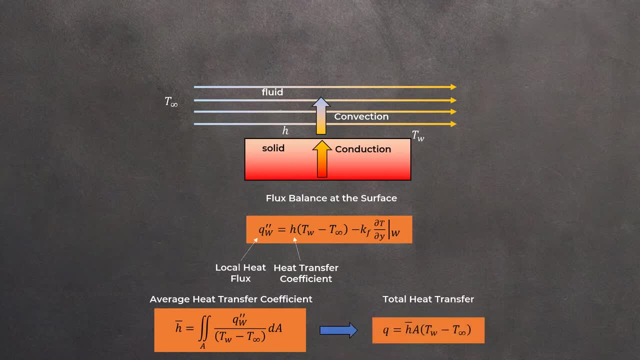 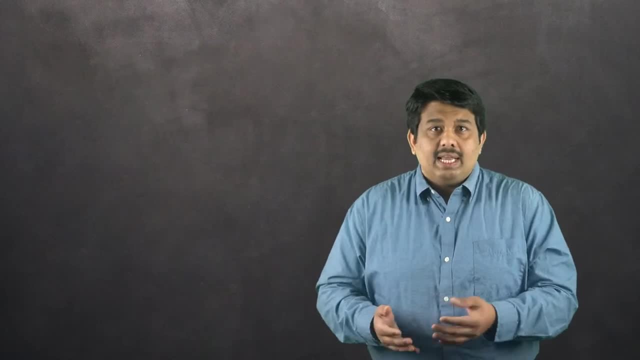 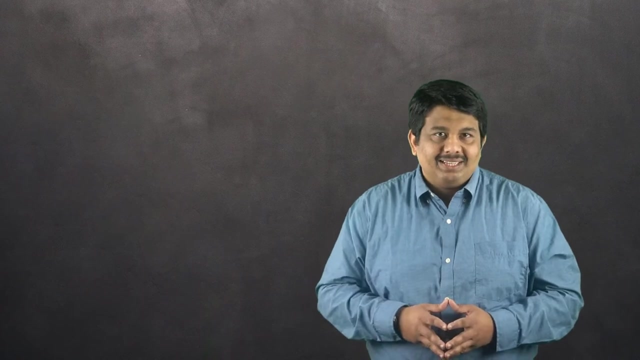 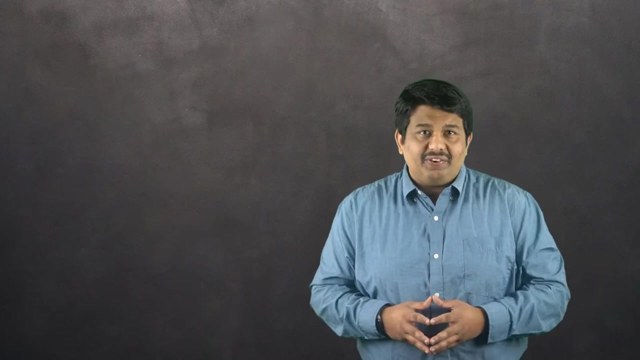 Subsequently, the total heat transfer rate is defined by the following relation: Note that H is always a positive number and therefore the sine of Q will depend on the temperature difference between Tw and T-infinity. The essence of any convection problem is determining the local and average heat transfer coefficients which can subsequently be used. 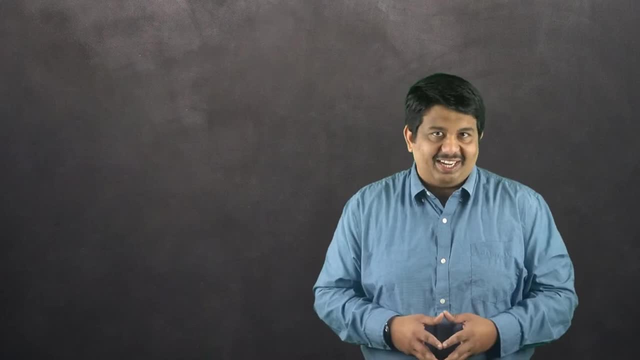 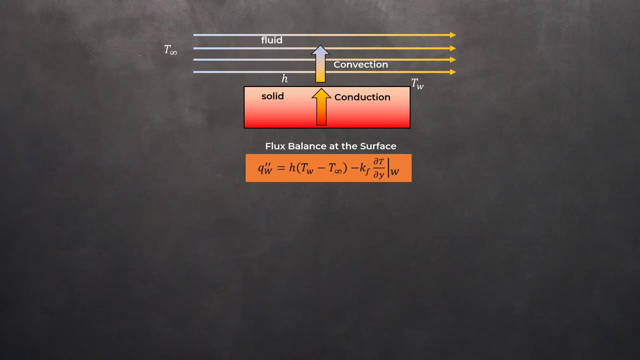 to calculate the local flux or the total heat transfer rate. Let's go back to the heat flux balance at the wall. If we now non-dimensionalize this equation using a reference length L and a reference temperature T-infinity, we get the following equation: 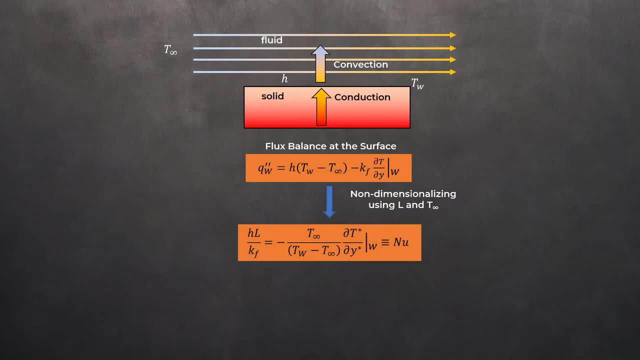 The heat flux balance can be rewritten as shown here. Note that Tw, T-infinity H and Kf are resumed to be constant. The circle term here is generally referred to as the Nusselt number. It is a non-dimensional measure of the convective heat transfer. 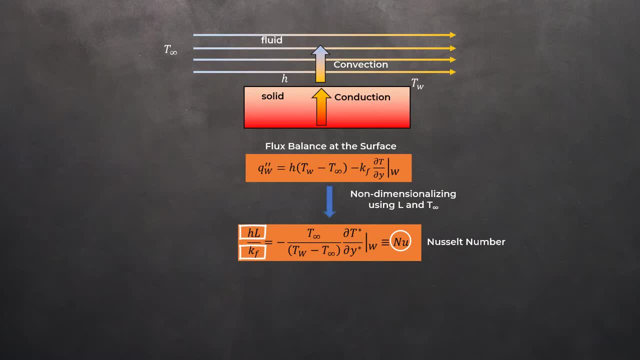 relative to the heat transfer that would occur by conduction into the fluid. If the heat flux balance is non-dimensional, the heat flux balance can be rewritten as shown here. The telling of T-infinity: EUÄÅÅ�uuøÅÎÅÄÅÅ×ÒÒ. 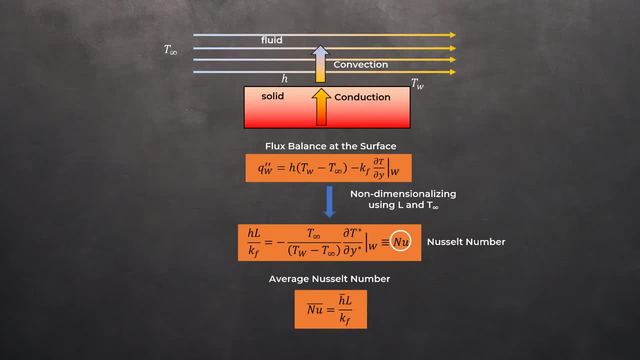 G is the its heavier temperature, which normally reacts with T-infinity. So if the majority of the keyword insgesamt is constant, as an expected result, then we should be able to heavier G andisini SiÅÆÄÅÅÒ·ÒÒÒÒÒÒÒÒÒÒÒÒôÒÒÒÒÒÒÒörÒÒÒÒÒÒÒ ÒÒord. 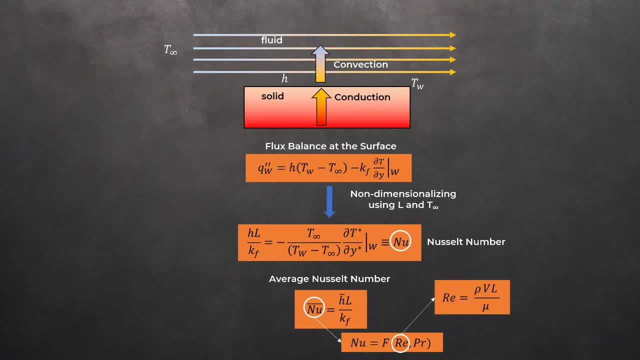 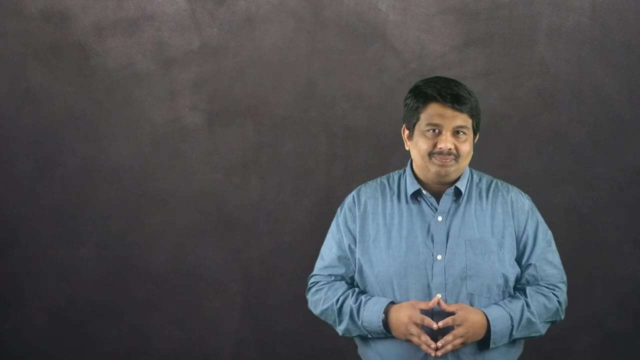 ratio of the inertial to viscous forces in a fluid flow and the Prandtl number, which represents the ratio of viscous diffusion of momentum to the thermal diffusion in the fluid. To determine the heat transfer coefficient, there are two ways: Through a series of experiments. 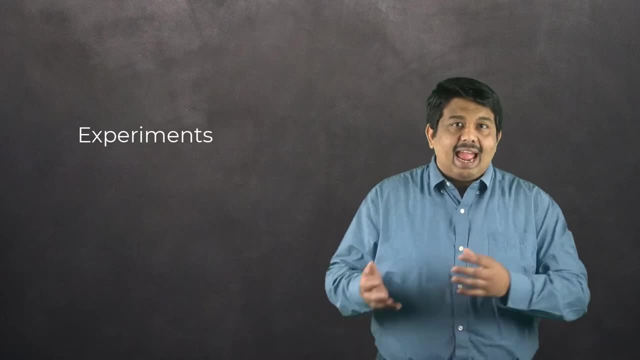 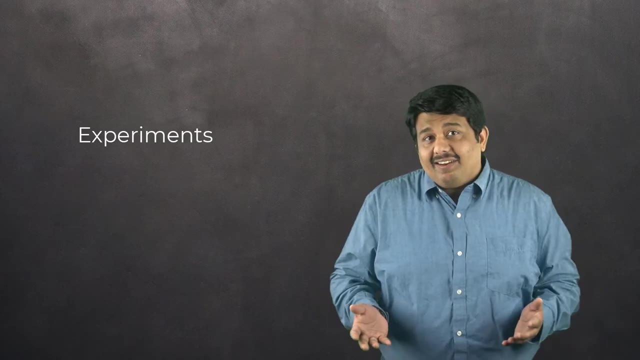 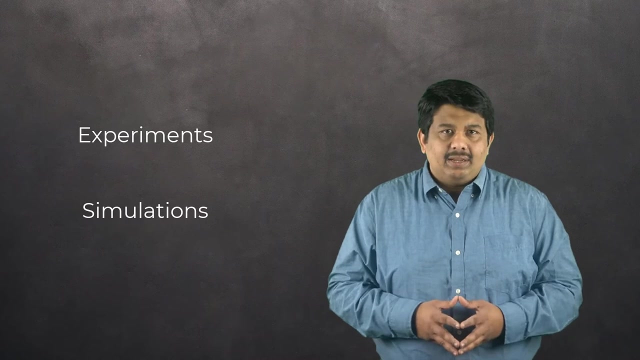 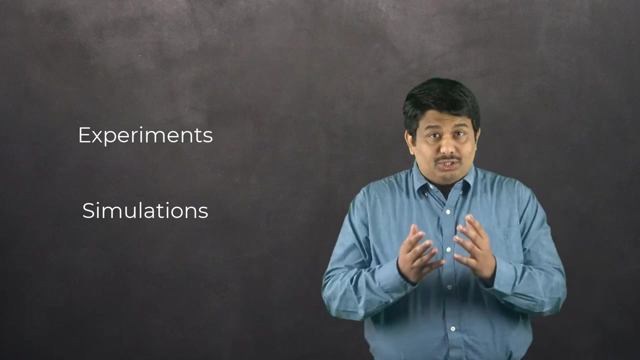 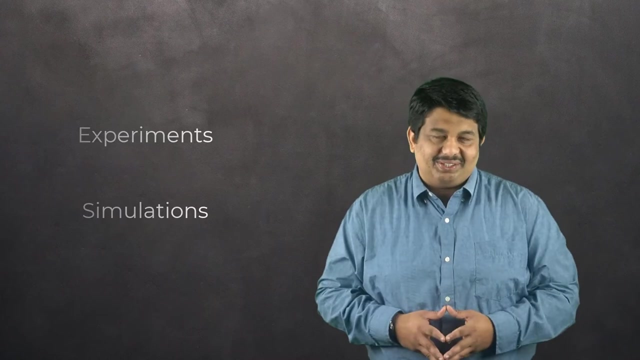 where key parameters such as geometric and thermal are varied and the fluxes are measured carefully. The second way is through simulations, wherein the governing equations are solved using CFD techniques for specific geometries and flow and thermal boundary conditions. This is akin to doing experiments, except now we are simulating the fluid flow numerically using computers. 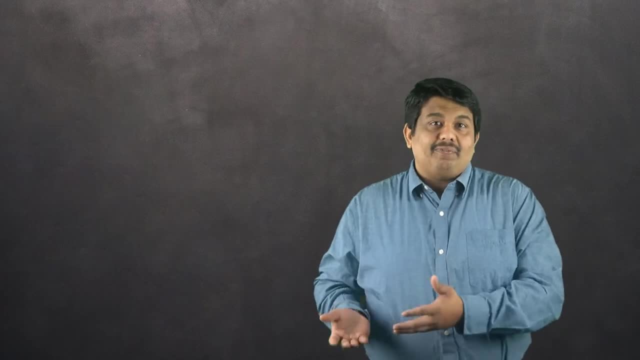 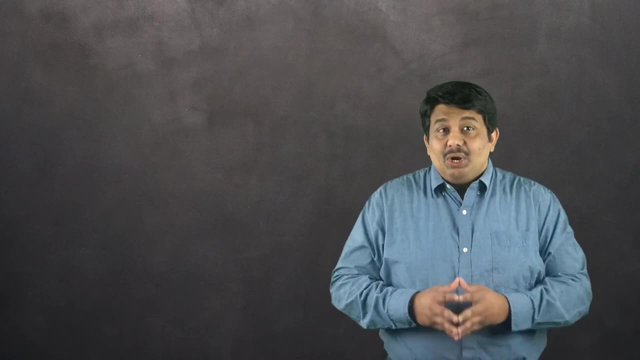 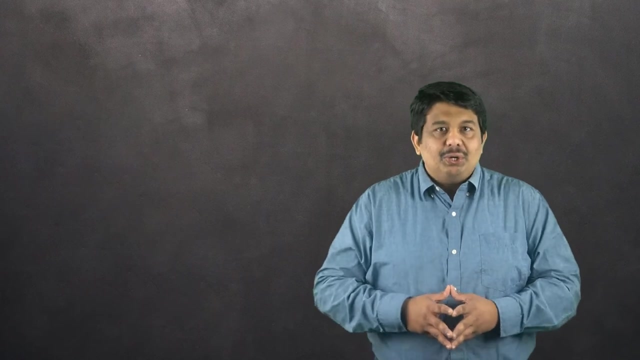 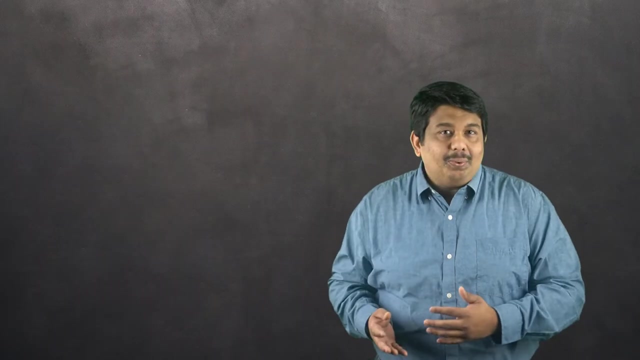 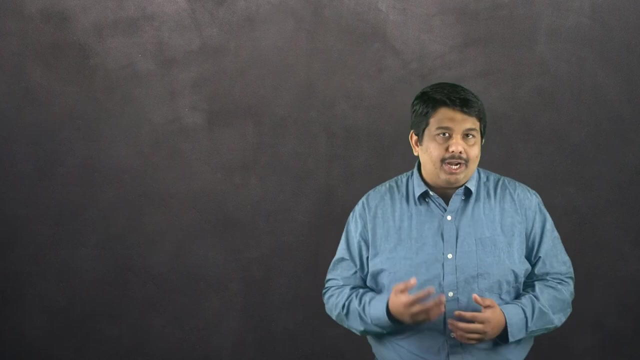 However, it is impossible to perform experiments or simulations for every conceivable geometry and flow condition. To address this issue, engineers make use of similarity methods and dimensional groups to develop correlations for common geometries and flow conditions. There are two types of similarities: geometric and dynamic. Geometric similarity means that two bodies are geometrically similar in both ways, as there are no convergence or gap between two bodies. What is difference between two bodies is the relationship between the two ways. The laws of mass transfer and the flow condition can be seen at a later point in. 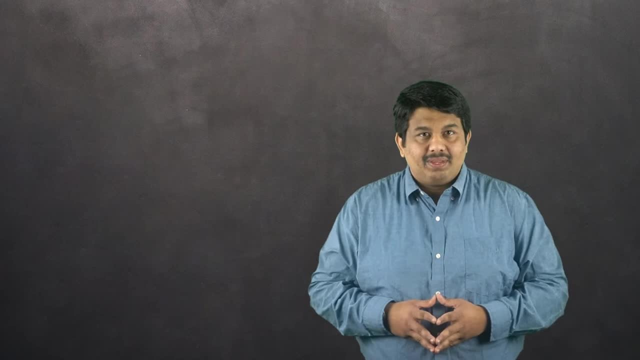 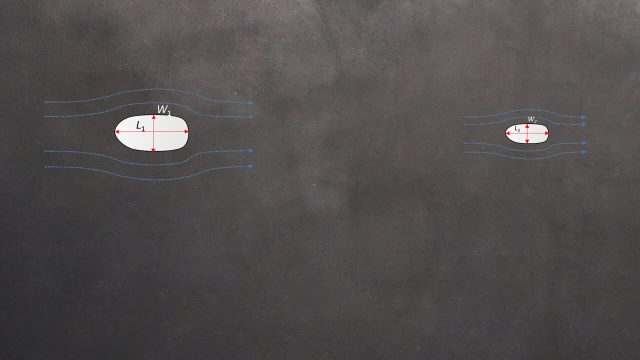 if they are perfectly scaled versions of each other. Consider the following two objects: If they are geometrically similar, then it is required that the ratio of corresponding lengths of the two objects, ie L1 over L2, W1 over W2, etc. are the same. 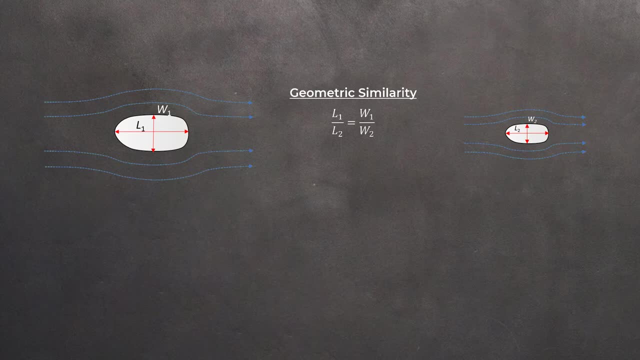 Dynamic similarity requires that for geometrically similar bodies the flow patterns are also similar, ie the velocities, velocity gradients, fluid forces and streamlines all scale. with the geometry For heat transfer problems it is also required that the temperatures, temperature gradients,